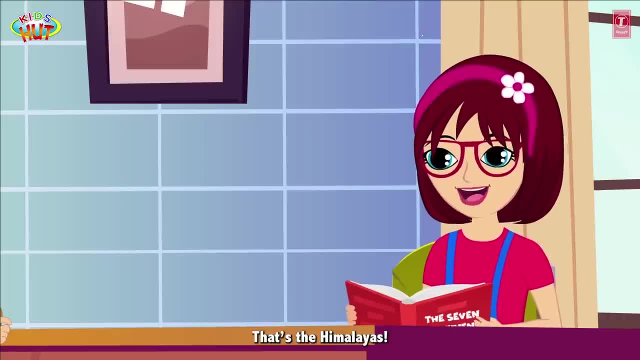 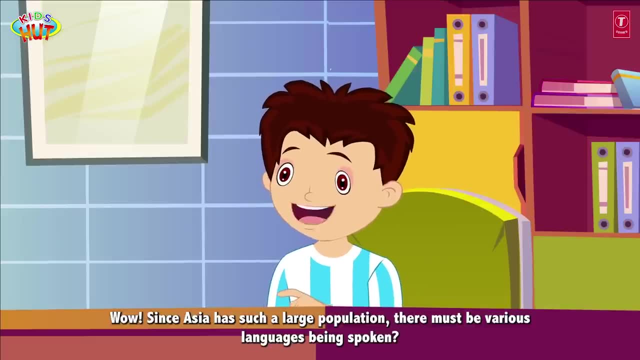 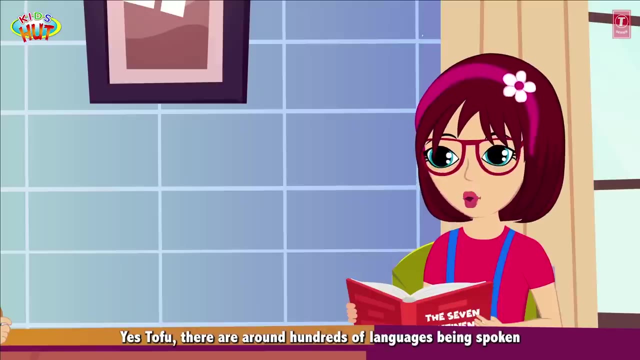 And what are those? That's the Himalayas. They are the world's highest mountain peaks. Wow, Since Asia has such a large population, there must be various languages being spoken. Yes, Tofu, There are around hundreds of languages being spoken. 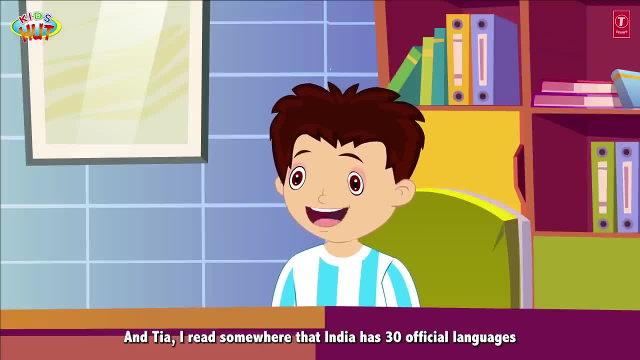 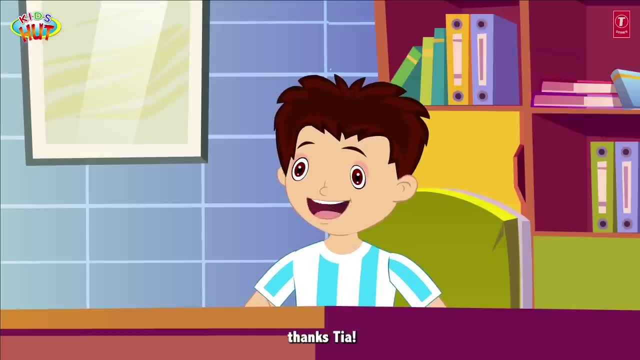 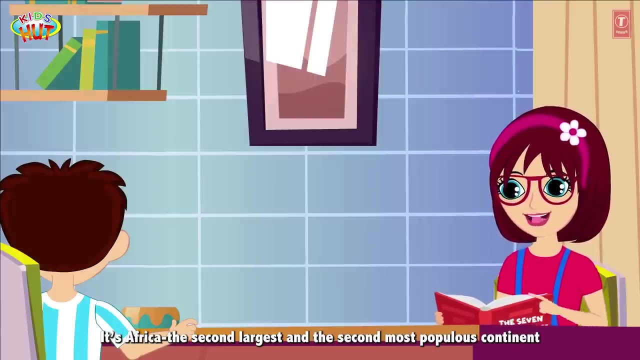 And dear. I read somewhere that India has 30 official languages. That's right, Tofu, You're pretty smart. Oh thanks, dear. What about the next continent? It's Africa, The second largest and the second most populous continent. 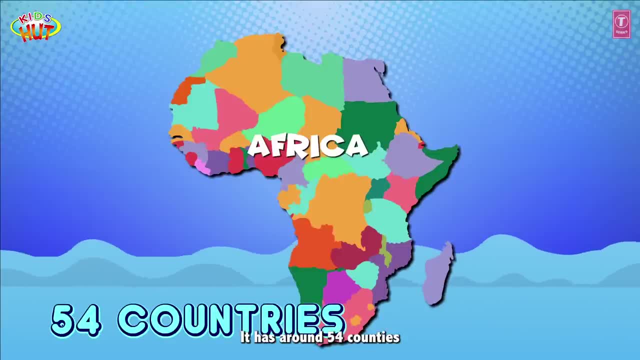 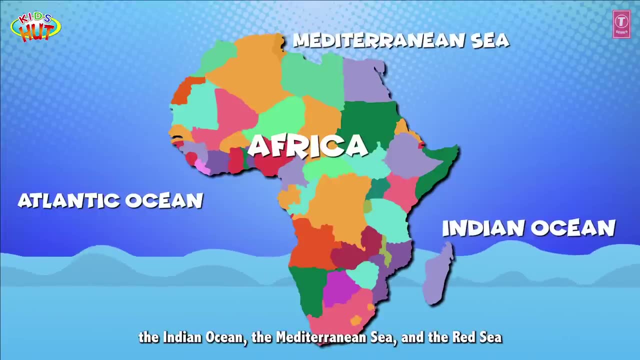 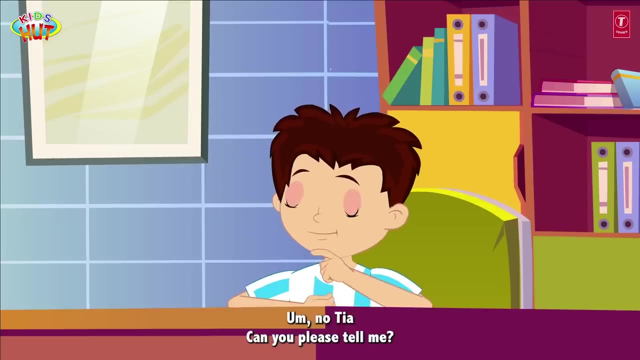 It has around 54 countries. The African continent is surrounded by the Atlantic Ocean, the Indian Ocean, the Mediterranean Sea and the Red Sea. Can you name the largest country in Africa? Hmm, No dear, Can you please tell me? The largest country in Africa is Algeria. 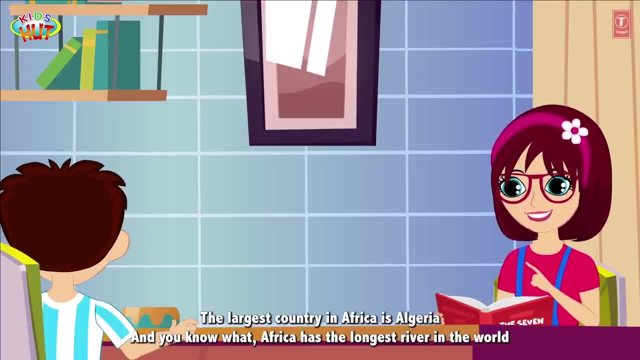 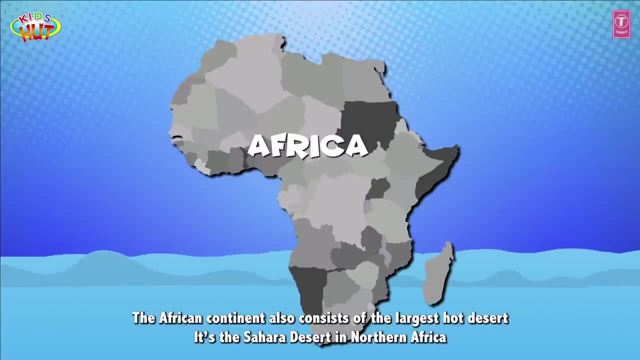 And you know what? Africa has the longest river in the world. It's the river Nile. The African continent also consists of the largest hot desert: It's the Sahara Desert in Northern Africa. Wow, Africans must be proud of having the longest river. 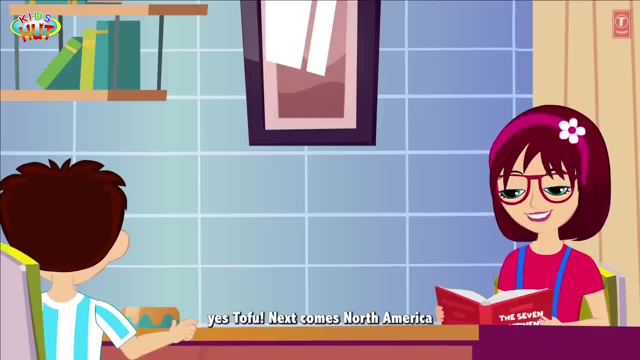 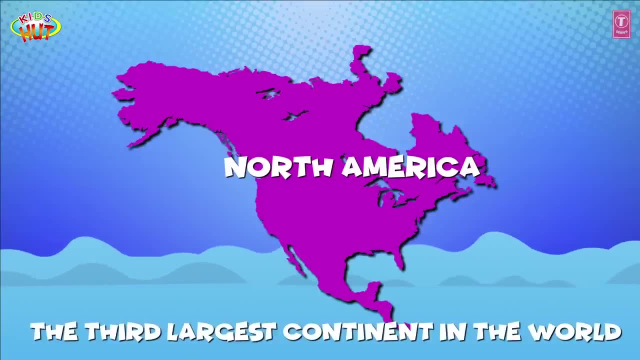 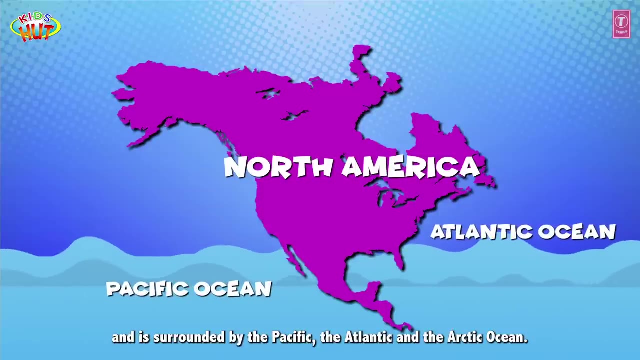 and the largest hot desert in the country, Yes Tofu. Next comes North America, the third largest continent in the world. North America has 23 countries and is surrounded by the Pacific, the Atlantic and the Arctic Ocean. Isn't USA North America? 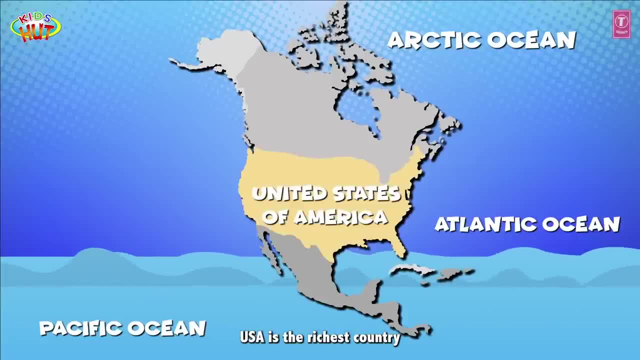 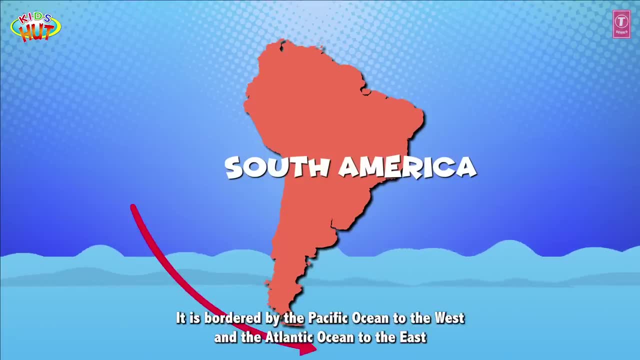 Yes, Tofu, USA is the richest country and Mexico is the most populous. Next comes South America. It is bordered by the Pacific Ocean to the west and the Atlantic Ocean to the east. South America has 12 countries. Wow. What is the next continent, dear?